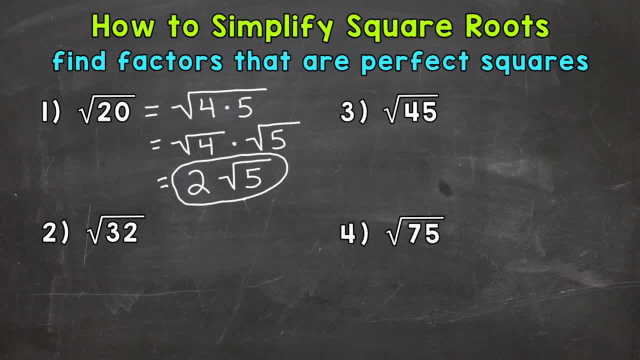 root 5.. Let's try another one and move on to number 2, where we have the square root of 32.. So we need to think: are there any factors of 32 that are perfect squares that are perfect squares, So any numbers that can go into 32, so to speak, that are perfect squares? If so, we can simplify. 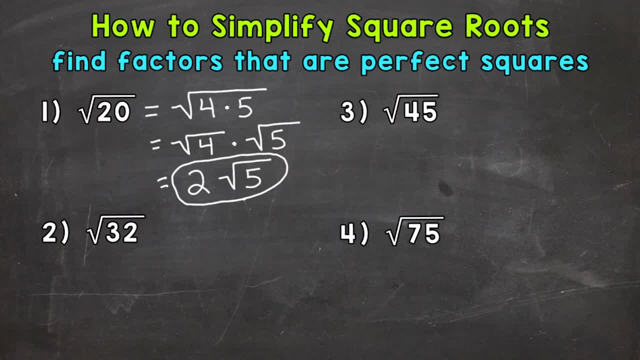 If not, it's already in simplest form. Well, we know that 16 times 2 equals 32, and 16 is a perfect square. so we can simplify: The square root of 32 equals the square root of 16 times 2.. Let's split. 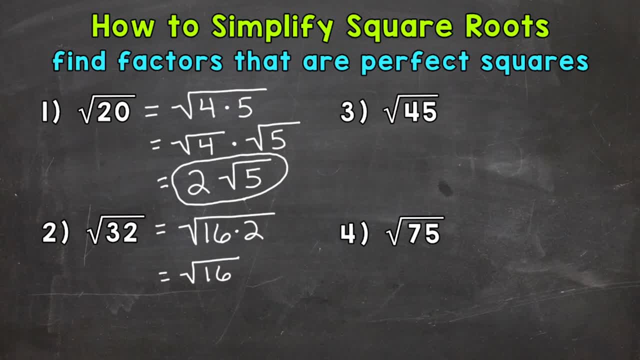 this. so we have the square root of 16 times the square root of 2.. 16 is a perfect square, so the square root of 16 is 4. so we end up with 4 times the square root of 2.. Or 4 square root 2 or you. 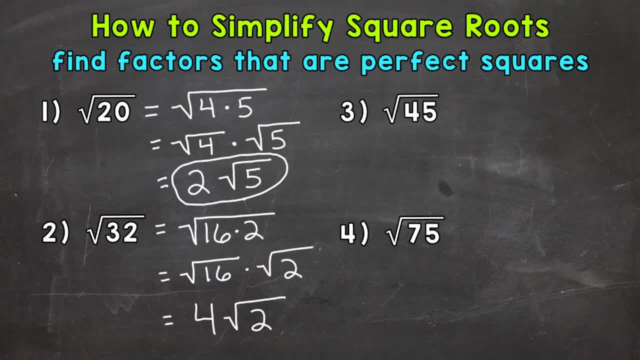 can even say 4 root 2.. Now, 2 cannot be simplified any further, So this is our final answer. As this is the final answer, I hope you've found it helpful. If so, leave a comment down below. Watch usundoGamescom. We'll see you soon, Bye, bye. 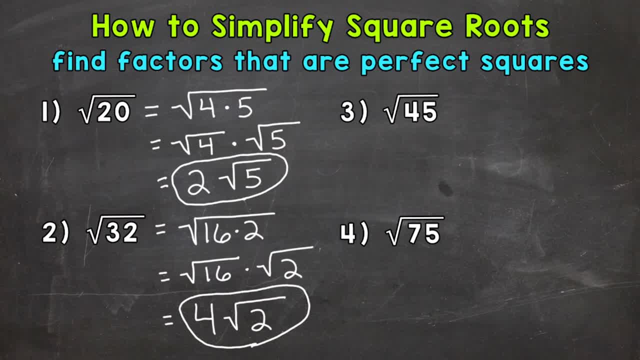 simplifying the square root of 32.. Now I do want to mention we can take another path to get to that same answer for number two. I'm going to try to squeeze it in to the left here. We know that 4 times 8 also equals 32, and 4 is a perfect square. So this is the other path we can take and I'm 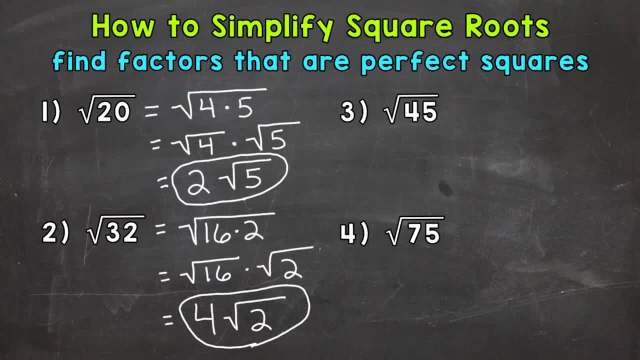 going to start by splitting these, just to make sure I have enough room. So we have the square root of 4 times the square root of 8.. The square root of 4 is 2.. Let's bring down our square root of 8.. Now we can continue to simplify. We're not done yet, because we have a perfect square within. 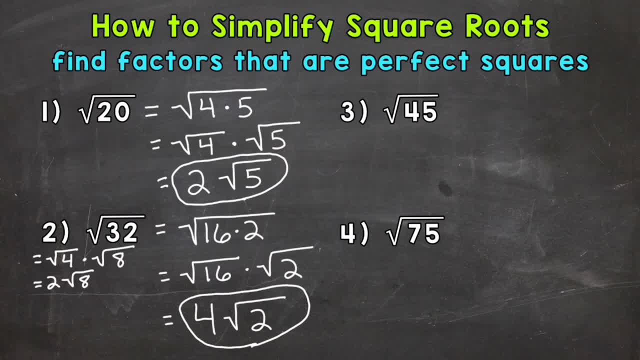 8 as far as factors go, because 4 times 2 equals 8 and 4 is a perfect square. So again we can continue to simplify. So we have 2 times the square root of 4 times the square root of 2.. So the square root of 4 again is 2.. So we end. 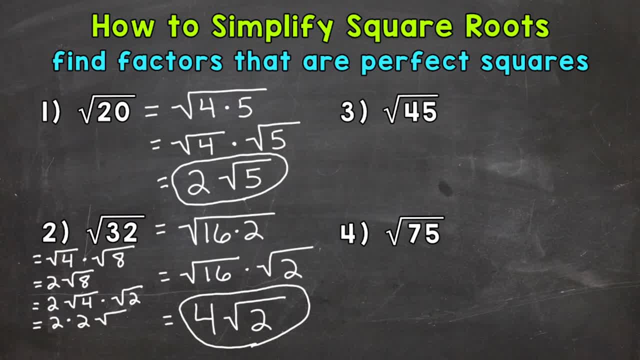 up with 2 times 2, times the square root of 2.. Now the square root of 2 is simplified, so we can't break that down any further, but we can multiply our 2 times 2.. So 2 times 2 gives us 4, and then 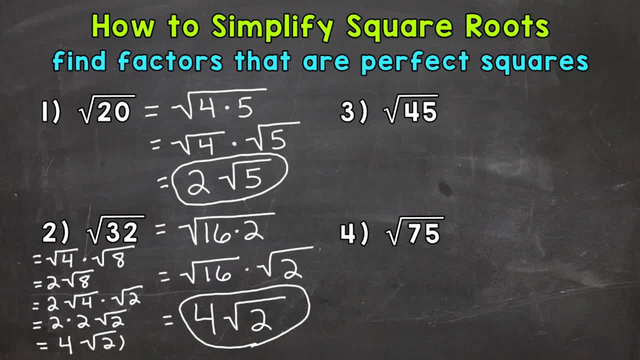 we have the square root of 8.. So we have the square root of 8 times the square root of 2.. of two, So same exact answer, but a different path. And that's okay. Both of those paths are correct, So keep that in mind. There may be different paths as far as simplifying a square. 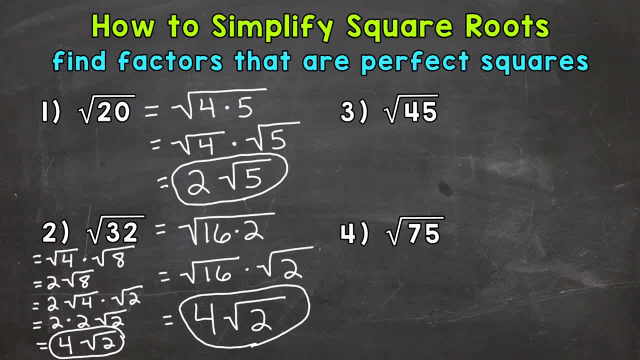 root. Just always remember to check if you can simplify further. Let's move on to number three and try another one where we have the square root of 45. So think any factors that are perfect squares. Yes, 9 and 5 are factors of 45.. 9 times 5 equals 45. And 9 is a perfect square. So the 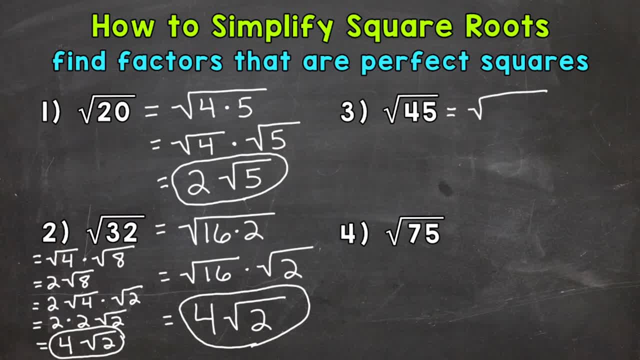 square root of 45 equals the square root of 9 times 5.. Let's split this. So square root of 9 times the square root of 5.. So the square root of 9 is 3.. Bring down our square root. 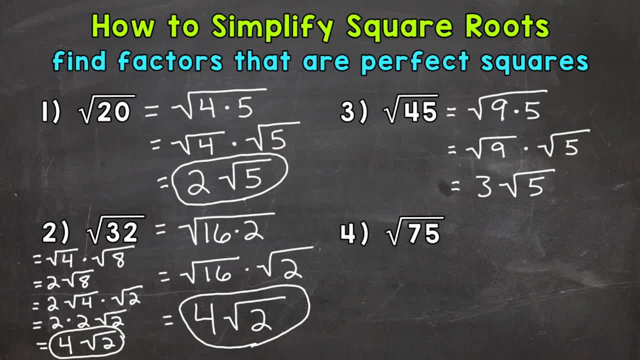 of 5.. That cannot be simplified any further. So we have 3 times the square root of 5, or 3 square root 5 or 3 root 5.. Lastly, number four, we have the square root of 75.. So any factors that are. 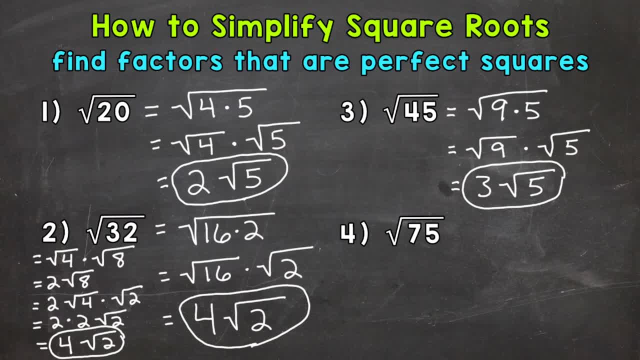 perfect squares. Well, 25 and 3 are factors of 75.. 25 times 3 equals 75.. And 25 is a perfect square, So the square root of 75 equals 75.. And 25 is a perfect square, So the square root of 75 equals. 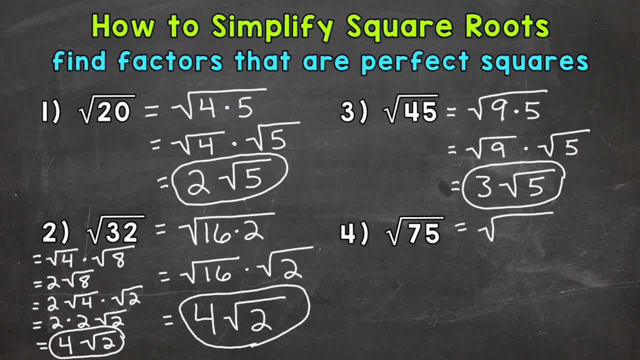 of 75 equals the square root of 25 times 3.. Let's split so we get the square root of 25 times the square root of 3.. Now the square root of 25 is 5, so we have 5 and then the square root.